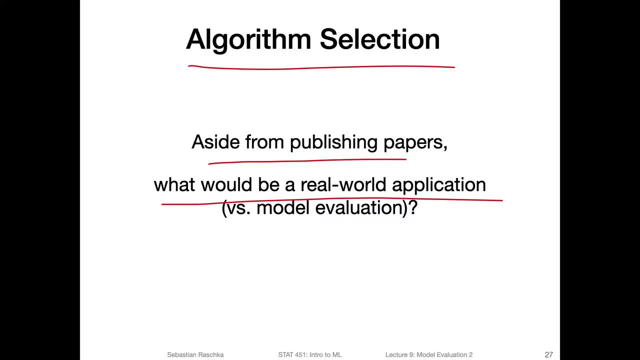 I I remember that I talked about a case where we developed, let's say, an email application And the email application has a machine learning algorithm that learns, based on the user behavior, to identify spam and non spam for that user. So in that case we 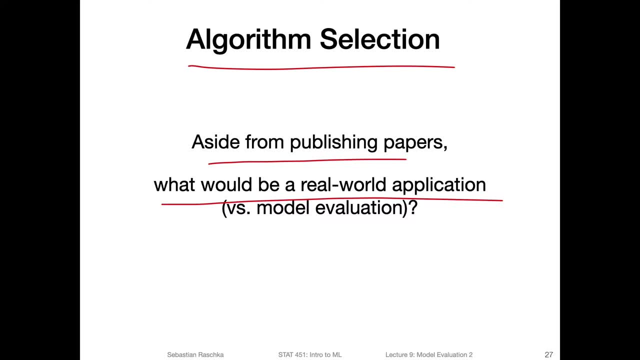 want to ship an algorithm that can learn well on email data, So we may want to compare different algorithms on different training sets and see which one performs best in the practical scenario. Another case would be on archive sanity. This is, I think it's called, archive sanity Preserver. 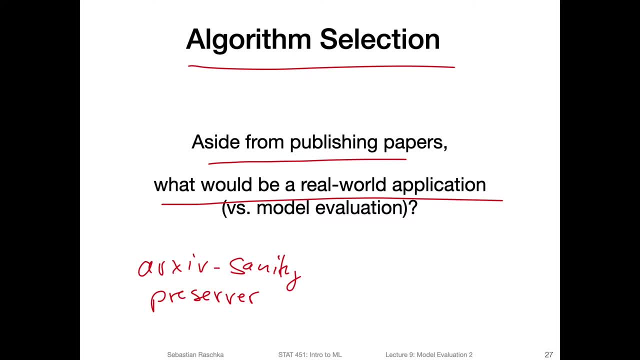 actually. So I don't remember right now the detailed or the exact web address, But if you search on that on the web, I think you will find it. So this is like a layer on top of an web application on top of archiveorg, which is a server for. 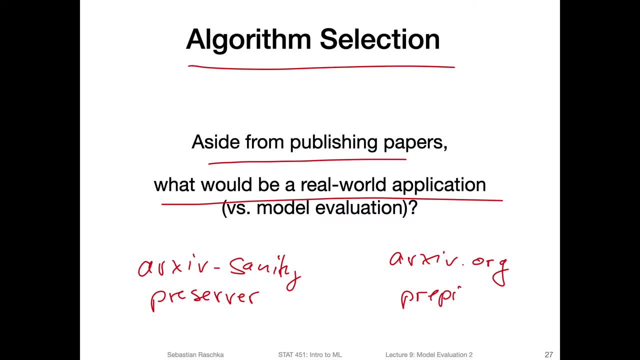 hosting preprints. So preprints are articles, So traditionally these are articles that have not been published yet or not been peer reviewed yet. So, for example, if you would write a paper and journal and or conference allows it, then you can post a early version of 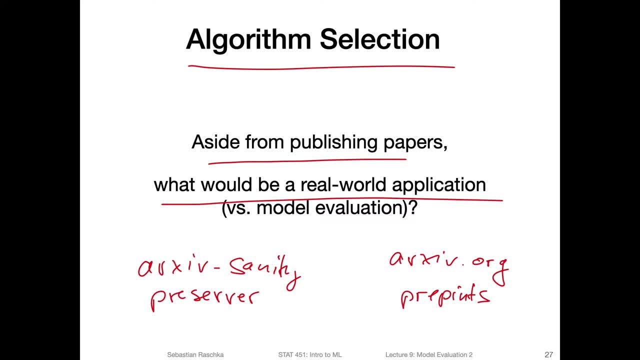 your article before it has been reviewed And before it has been accepted. Nowadays, it's also sometimes common to post a preprint, like a manuscript version, after the article has been accepted or after the article has even been published. So this is usually so that other people can access the article. 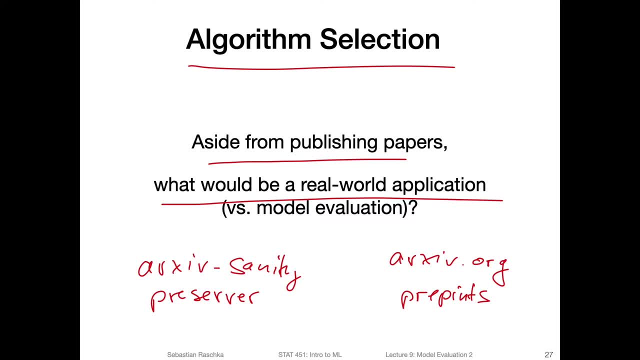 because sometimes it takes a while until after acceptance, until the article is published. it's in the conference proceedings And some journals. they charge substantial amounts of money for accessing an article, So not everyone has, let's say, a subscription for that journals And that way people who don't 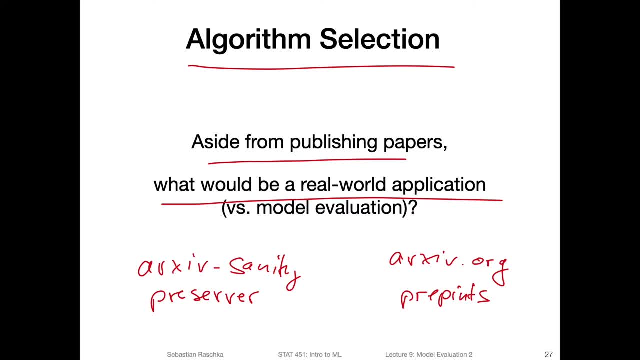 have a subscription can also read the article for free. But yeah, so archive. we have actually a lot of preprints every day, like hundreds of machine learning papers And one of the moderators- they're like helping- taking a look at whether the submissions look good And it's. 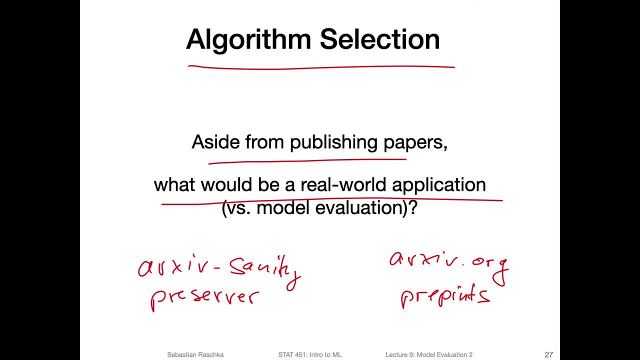 actually a very interesting thing to do because you see all the interesting titles every day uploaded, So you get an idea what's currently trendy in machine learning or machine learning research, but we usually have around one to 200 articles each day And the archive sanity preserver is a. 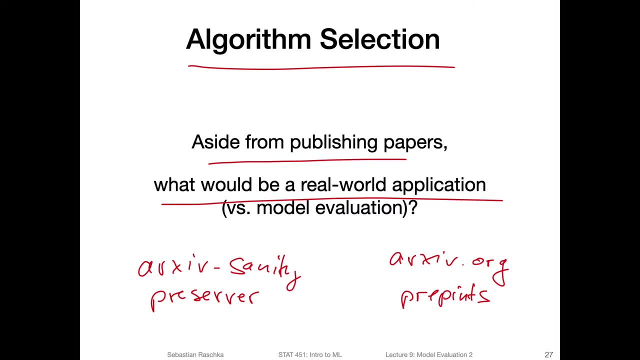 web application. I think it's developed by Andre Kapathy And it uses a support vector machine for each user that you can create an account. So support vector machine learns from papers you like, so you can like papers and search for similar papers And the support 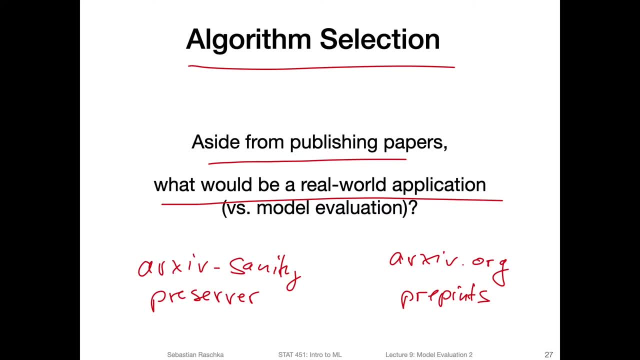 vector machine is one for each user. it will learn from your behavior and then make recommendations of articles you might be interested in. So in that case, here it was also important to select a good algorithm that is maybe fast, but then also accurate when it learns from the user behavior. 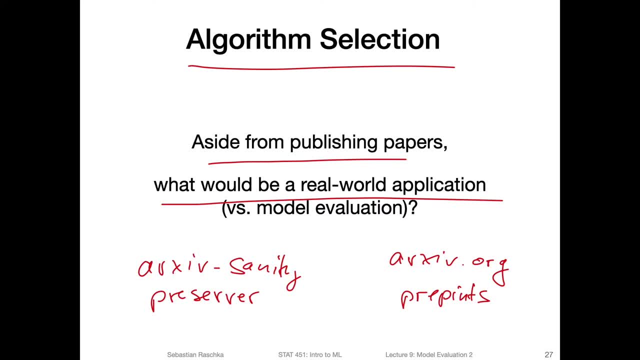 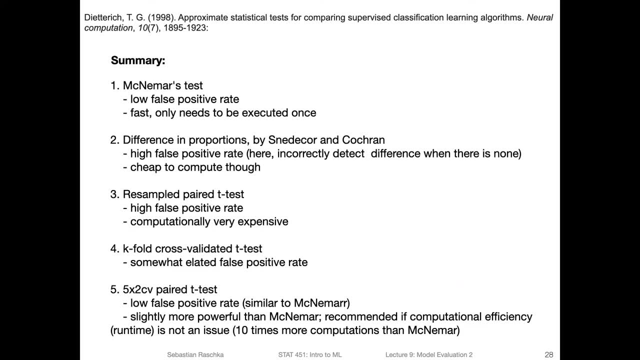 So there would be a case where algorithm selection would be an interesting topic for development. Okay, so that was a long speech, So here is an overview of different techniques, such as the tests. So it's a paper by Tom Dietrich, who is also one of the moderators on archive. So 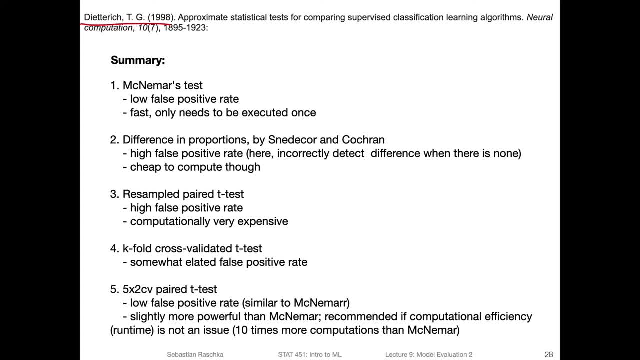 the articles are already 20 years old, But it's still a good summary because these are, I would say, the major techniques you would think about if you have taken other statistical statistics classes and you wonder: can we apply this statistics test? 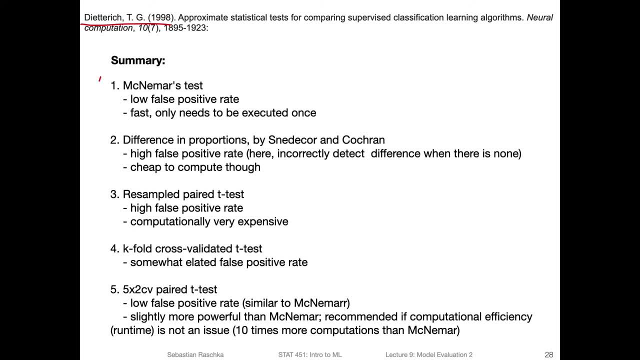 To machine learning. So McNamara's test- we talked about that before- this is actually not an algorithm comparison test, it's just a model comparison test, But so interesting to list here because, based on the study on empirical experiments, Tom Dietrich found that it has a low 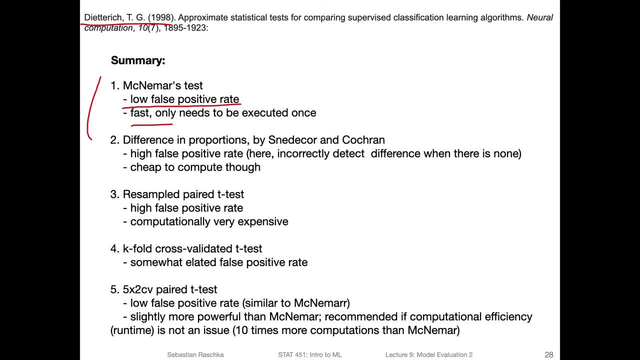 false positive rate, And it's actually also fast to run, which is nice if we compare two models to each other. There are other tests, for example the difference in proportions test. it has, unfortunately, a high positive rate though tests that require. 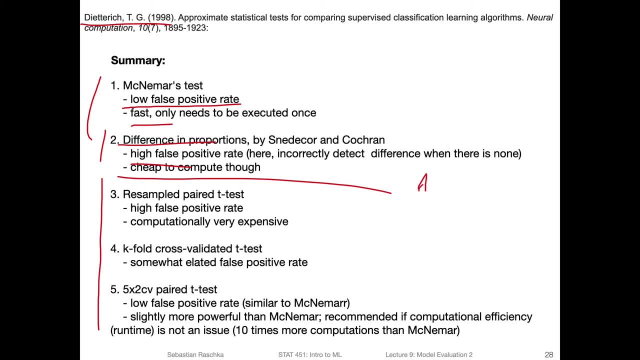 fitting multiple models. So this would be more the case for algorithm selection or comparison. at least let's call that algorithm comparison here These ones. they require fitting multiple models, but if they are more accurate they're actually quite useful. So here this one. unfortunately, the result is: 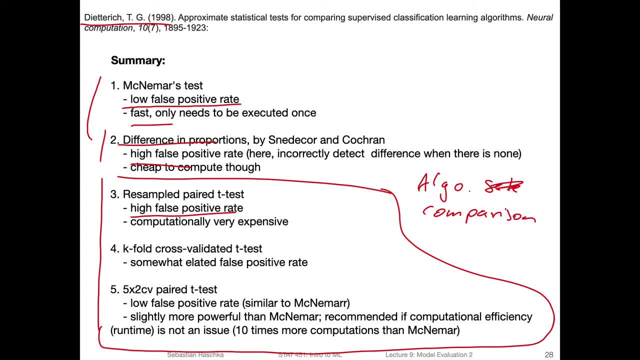 for example, pair t test has a high false positive rate And, similar to the repeated holdout method, it can be computationally expensive because we have to fit it to multiple training sets. A better method is the K forward cross validated t test. But 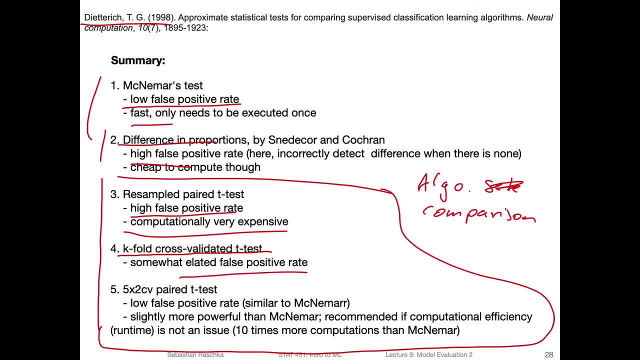 unfortunately it also has a slightly elated false positive rate, So with that wrongly rejecting the null hypothesis even though the null hypothesis is true. And another method is the five- two cross validated paired t test. This is a technique that was proposed in this paper And this one has a low false positive. 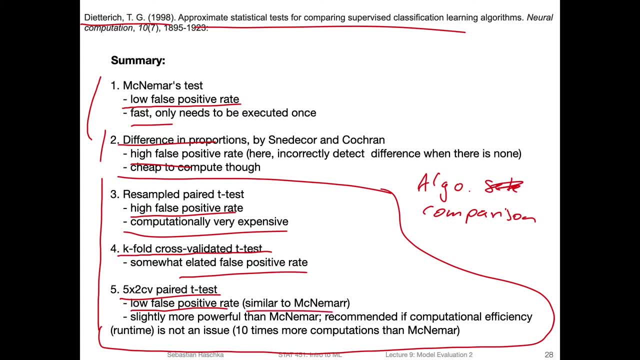 rate. So that is nice. It's similar to McNamara's test And it's a little bit- even a little bit lower, I think. And what's also nice, it's slightly more powerful than McNamara's test. So statistical power would be not reject, So rejecting the null. 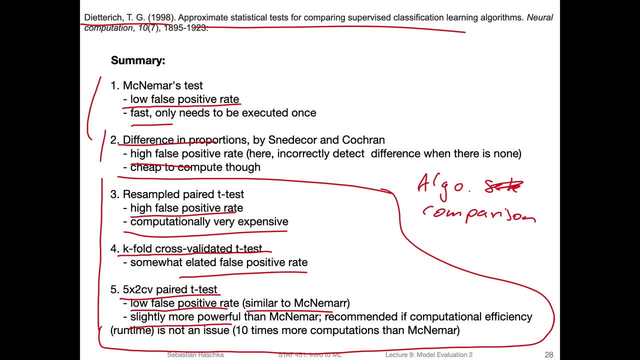 hypothesis. if the alternative hypothesis is true, so correctly rejecting the null hypothesis, So kind of detecting that there's a difference. So correctly detecting the difference, that would be the statistical power. Yeah, and this one would be one nice test to consider. There are 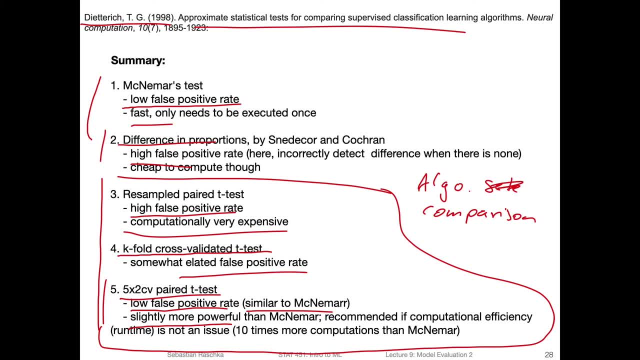 some newer, better approaches. For example, there's also a five times two CV paired f test, or sorry, not a parent parent f test, we can call it like that. So yeah, there are also other methods. I have written about this a little bit more in the 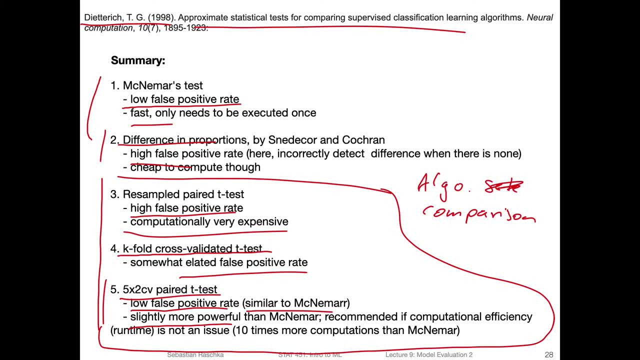 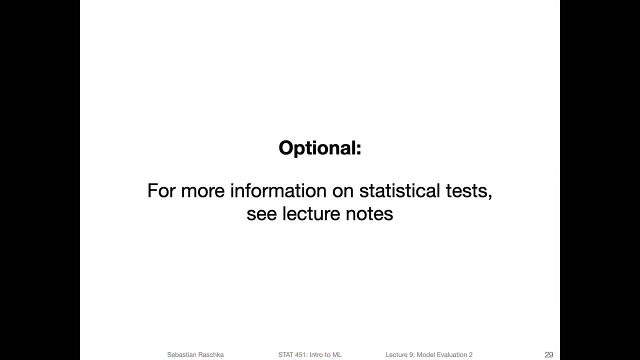 lecture notes. So, like before, we want go into all the details about all the statistical tests, But for those who are interested in that can read the lecture notes. And that's what I'm saying here. And also I implemented most of. 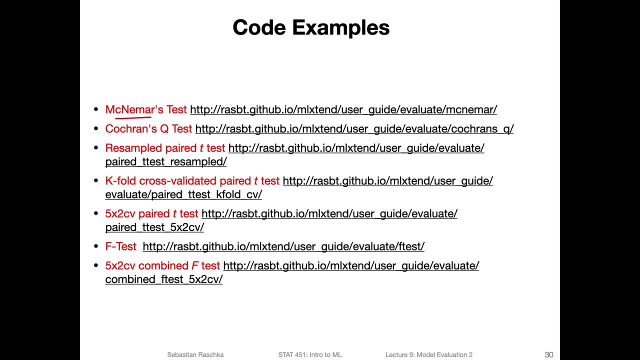 them in ml extend. So the McNamara's test, Cochrane skew test, the resampled PET test, which is actually not recommended But for educational purposes I implemented that here- the K fold cross validated PET test five times to CV PET. 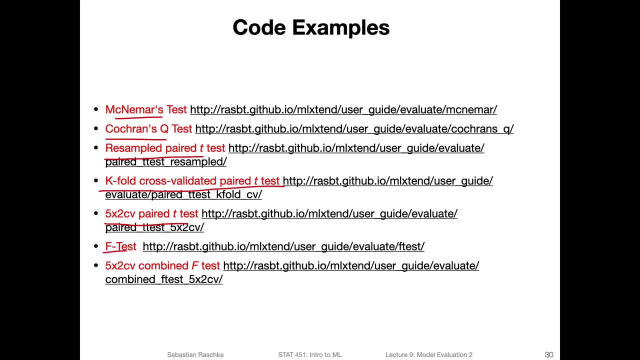 test recommended in. Tom did Rick's paper: regular F test and also the five times to CV combined F test. That's that's. I would say I improved version over the five times to CV parity test. So no, I put this one in here, probably a copy pasting, So I would.